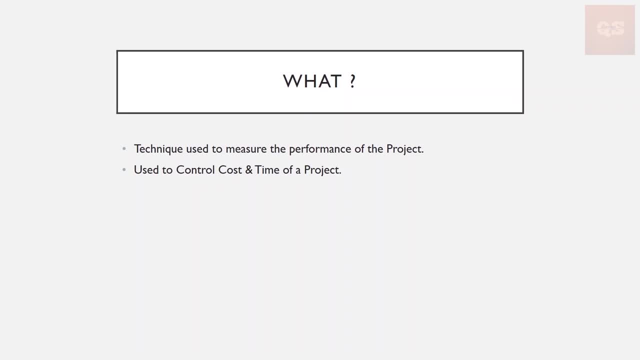 idea in the coming lectures where you will understand the different terms used in Earned Value Management, the formulas that is used, And I will also be sharing some scenarios wherein, using the different formulas, you'll be calculating whether the project is going as per the budget and as per the schedule. Now let's get to know the different terms used in. 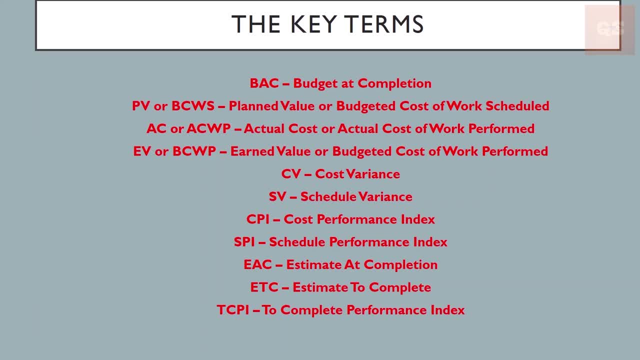 Earned Value Management. First we have the BAC, or the full form of which is called Budget at Completion. Then there is PV or BCWS, which is Planned Value or Budgeted Cost of Work Scheduled, Then AC or ACWP, which is Actual Cost, or also called as Actual Cost of Work Performed. Then we 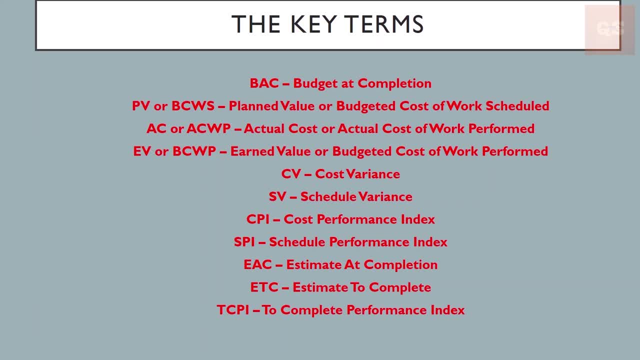 have the CV, which is Earned Value or Budgeted Cost of Work Performed. Then CV, which is Cost Variance, The SV, which is Scheduled Variance, CPI, which is Cost Performance Index. Then we have SPI, which is Scheduled Performance Index, EAC, which is Estimate at Completion. 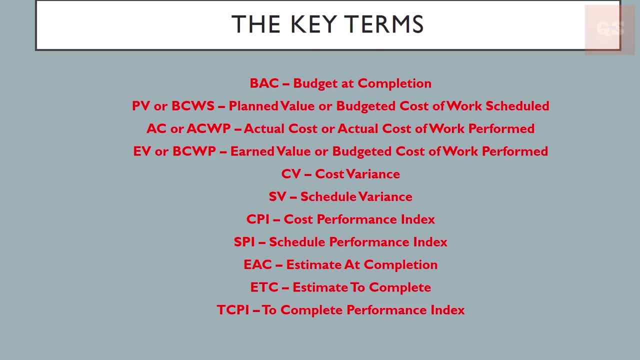 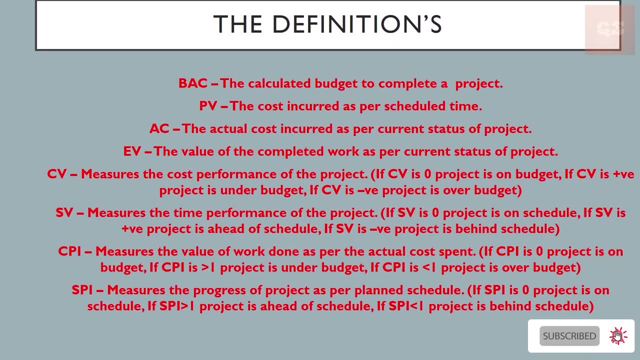 ETC, which is Estimate to Complete, And finally, TCPI, which is called to Complete Performance Index. The Budget at Completion is the calculated budget to complete a project. So, before starting a project, your estimation and tendering team will be carrying out and 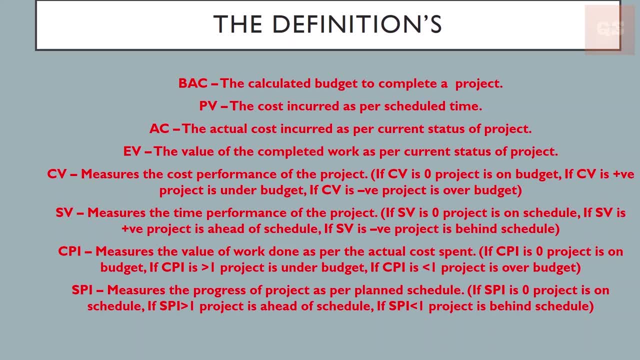 study to find out the cost to complete the project. This is basically the BAC. Then we have the PV or the Planned Value. This is the cost that is incurred as per the scheduled time. Basically, if 50% of your time is completed, that means 50% of your cost needs to be incurred. 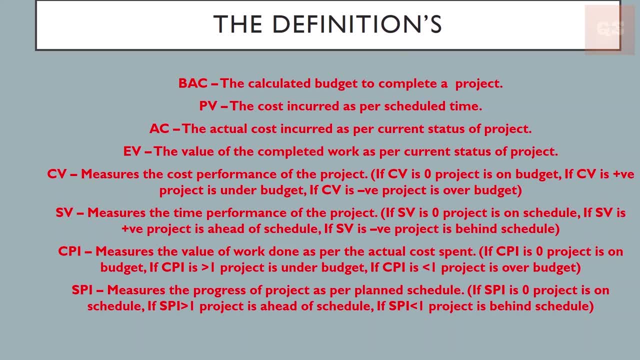 So this is the ideal situation. So this is called the Planned Value. So the actual cost is the actual cost that is incurred as per your current status of the project. So basically, if 50% of your work must have completed, but then the amount? 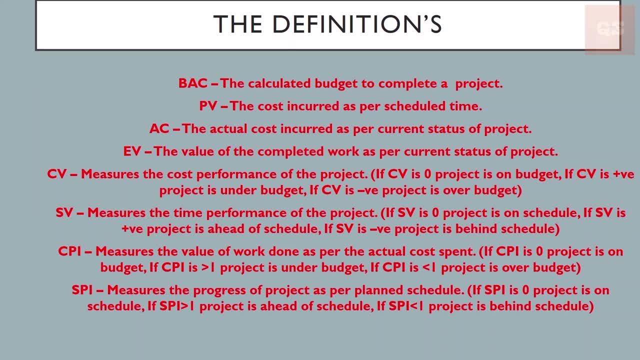 that you have incurred as expenses would have would be lesser or greater than your planned value. So this is basically the actual amount, or the correct amount that is being incurred as per the current status of the project. Next we have the Earned Value, The Value of the. 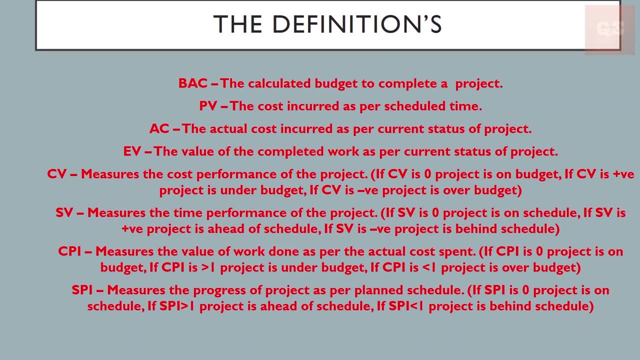 completed work as per current status of the project. So if 50% of your time is over but 20% of the work is completed, then the cost equivalent to that 20% of the work is called your Earned Value. Next we have the Cost Variance, which measures the cost performance. 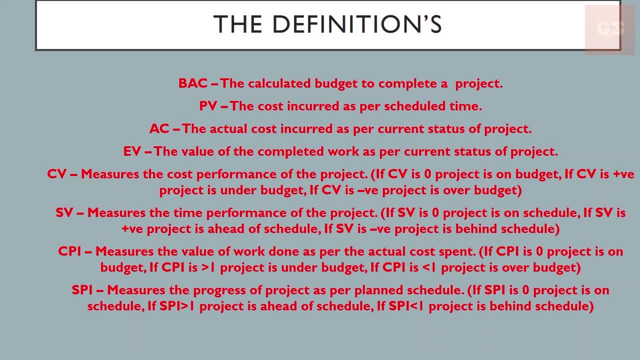 of the project. So if the CV is zero- using the formula when you find out the CV- and if it is zero, that means your project is on budget. If it is positive, that means the project is under budget And if it is negative that means the project is under budget And if it is negative, then 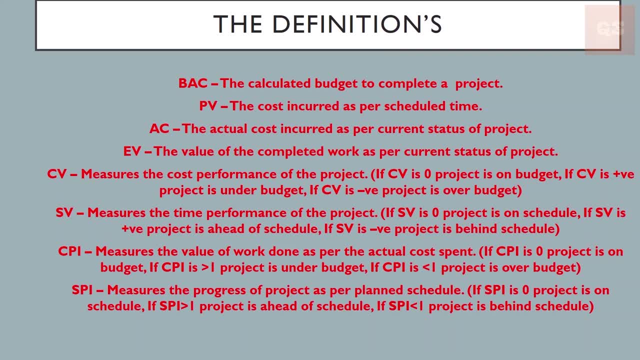 negative, that means the project is over budget. then schedule variance measures the time performance of the project. so if schedule variance is zero after calculating it, then it means that your project is on schedule. if it is positive, that means the project is ahead of your schedule and if it is negative, the project is behind schedule. then we have cpi. cpi and cv are almost. 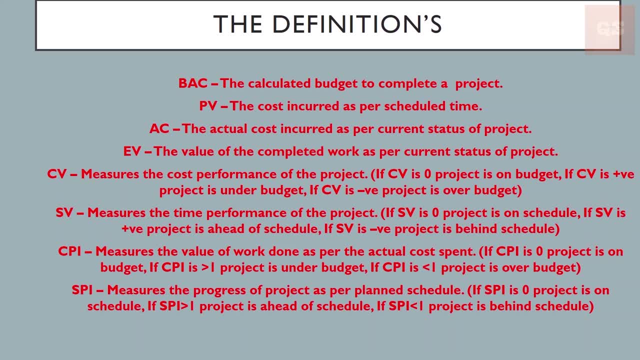 same, but cpi is the ratio and cv is the variance. the cpi is measures the value of work done as per the actual cost spent. if cpi is zero, the project is on budget. if it is greater than one, the project is under budget, and if cpi is less than one, the project is power. 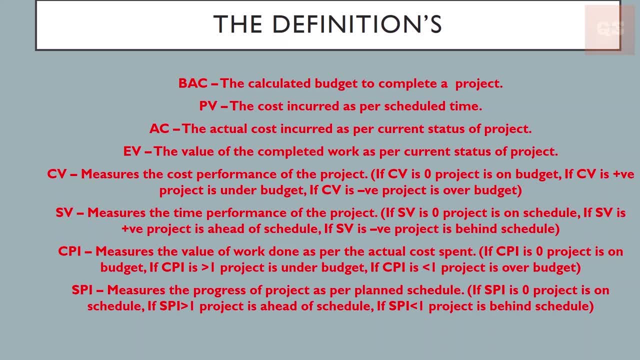 budget, then spi. spi and sv are also similar. again, spi is a ratio and sv is a variance. spi measures the progress of the project as per your planned schedule. so, after calculating, if spi is 0, the project is on schedule. if spi is greater than one, the project is ahead. of schedule and if spi is higher than alsoagar, the project is above schedule. then you set those values and cpi is greater than 1, which is more favorable for you, and you see the contract PV works on schedule, which we call supply margin, doesn't lag on budget. so this: 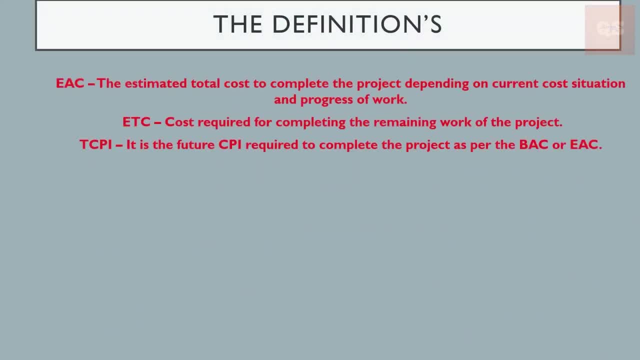 is the project we are pursuing, the final contract, which may vary when speaking right. so if cpi less than when the project is behind schedule, Then you have the EAC or estimated completion. So this is estimated total cost to complete the project, depending on the current cost situation. 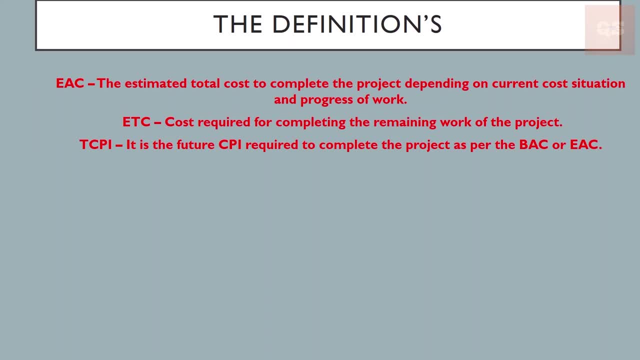 and progress of work. So sometimes your project will be not completed as per the BAC or your budget at completion. It might exceed the BAC or it might come less to the EAC. So the final cost to complete your project is called your estimate at completion. Estimate to complete is the cost. 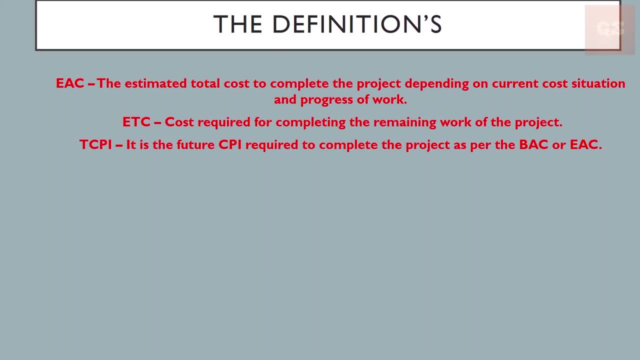 required for completing the remaining work of the project. So if your 80 percentage of work is completed and if you are asked to find out the ETC, that means what was the cost required to complete the remaining 20 percentage of work? That is called ETC, So TCPI is to complete performance index. So 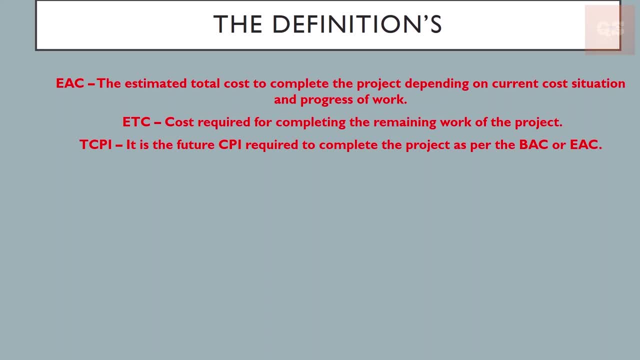 it is the future CPI that is required to complete the project as per the BAC or EAC. So if 70 percentage of your project is complete, now to complete the remaining 30 percentage as per your budget at completion or as per your estimate at completion, what is the cost performance index required? That is basically called the. 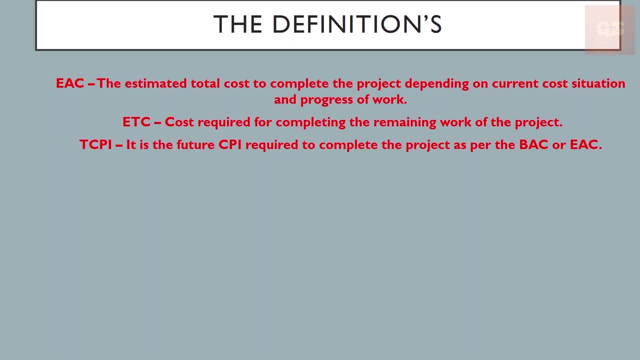 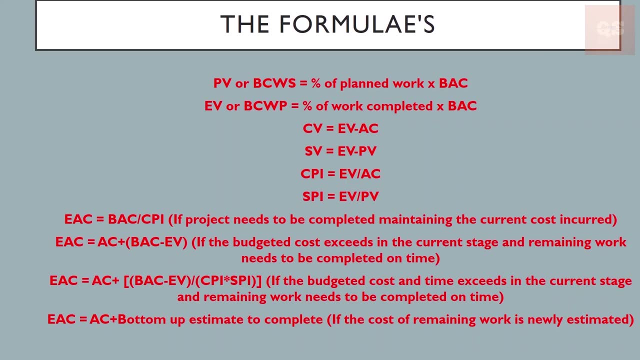 TCPI. So when you get to know the formulas and when we see the examples, you will have a better clarification on these definitions. Now let's look into the different formulas that is used to calculate the different elements of earned value management. First, PV or your budget cost of work. 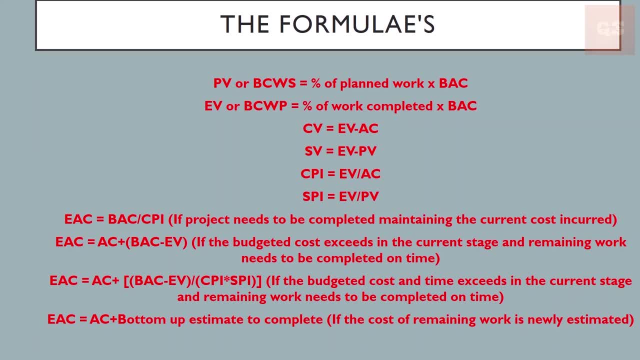 schedule. This is the percentage of the planned work into your budget at completion. So that's 50% of your work. your planned work is completed and then 50% into your budget at completion will give you your planned value. Then we have the EV or BCWP. So this is the percentage of the work. 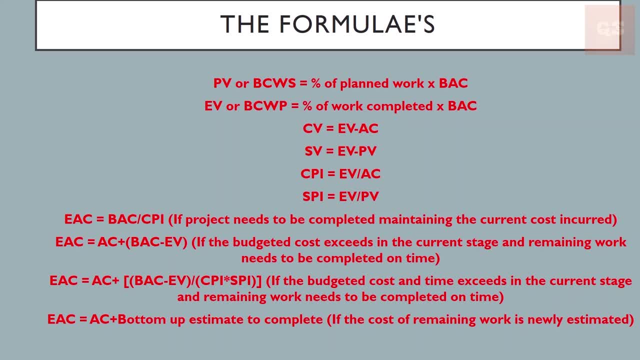 completed into budget at completion. So if halfway of through your project only 20% of the work has been completed, then that means 20% into the budget at completion will give you your earned value or BCWP. Next we have the cost performance index. So this is the cost performance index. This is: 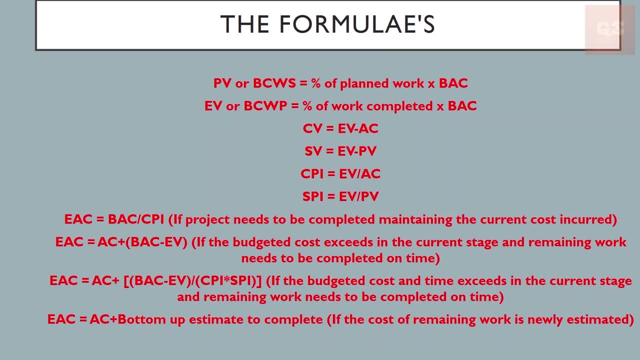 the cost variance, which is equal to the earned value minus actual cost. The schedule variance is equal to earned value minus the planned value. CPI or the cost performance index is equal to earned value divided by your actual cost. Scheduled performance index is equal to the earned value. 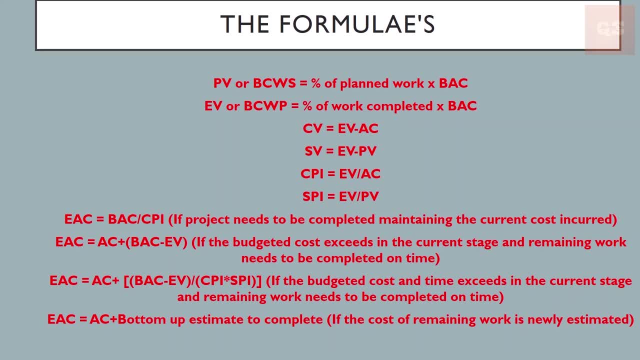 divided by the planned value. Next, the estimated completion. There are three situations to calculate your estimated completion. First one is when your project needs to be completed, maintaining the current cost incurred. If your current cost incurred is less than the current cost incurred, then 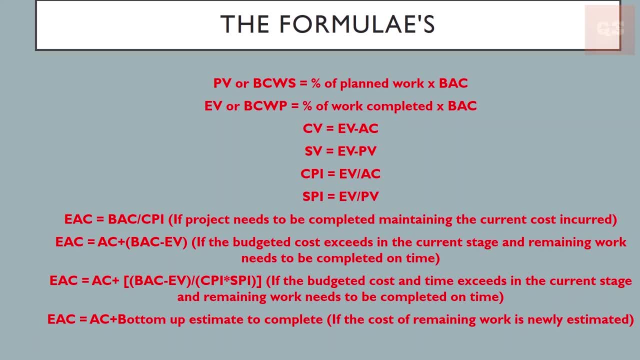 you need to calculate your CPI and the current situation, And if you need to complete the project in the same CPI, then your estimated completion will be equal to your budgeted completion divided by your cost performance index. Now, if you want to complete your remaining work on time, so at the 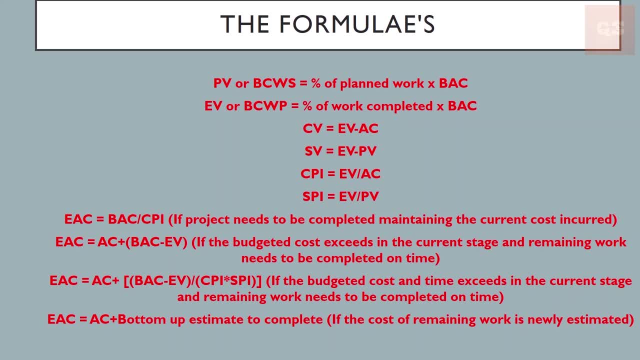 current situation, if the budget of the budgeted cost has exceeded and for remaining works you need to be calculated on schedule time. For that, your estimated completion will be equal to your actual cost plus the budgeted completion, minus EV. The next scenario is if the budgeted cost and also 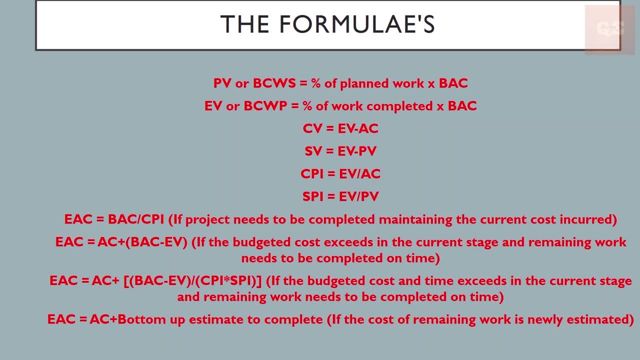 the time has exceeded in your current situation and the remaining works needs to be completed on time. For this scenario, your EAC will be equal to your actual cost, plus BAC, minus EV, divided by the cost performance index into your scheduled performance index. Next scenario is if the cost of the 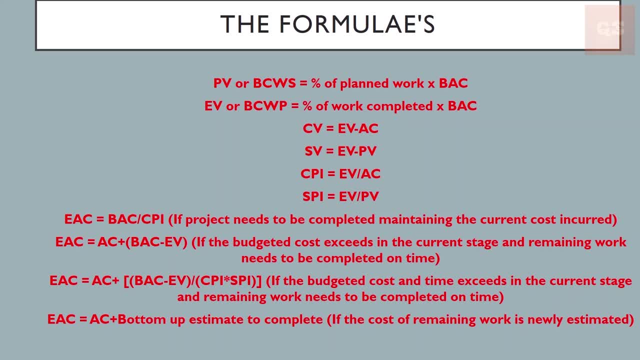 remaining work needs to be newly estimated. So the current cost is equal to the estimated completion of the remaining work. So in this current situation, you have found out that you have incurred this much cost. So you are going to estimate your remaining work freshly. But in that scenario, your estimated 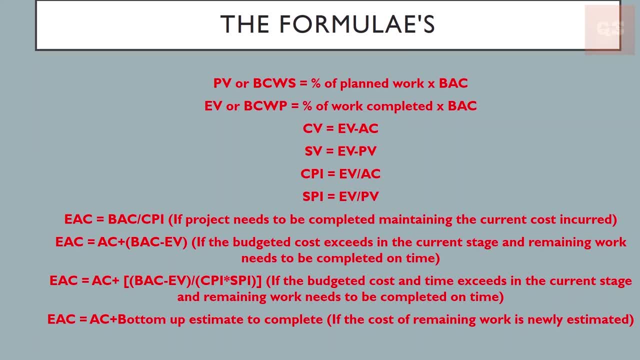 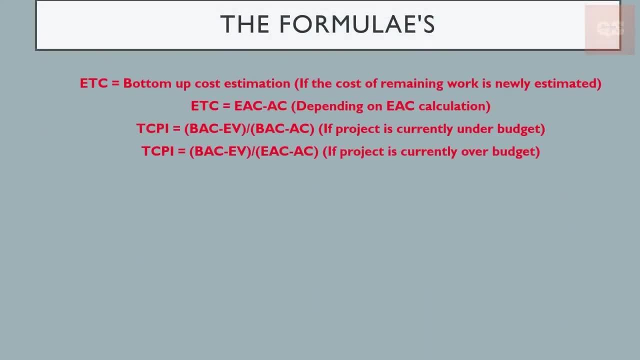 cost will be equal to your actual cost that has been incurred till date, plus your newly estimate to complete the remaining part of the work. So the bottom up estimate to complete. Next is your estimate to complete, So the remaining the cost required to calculate the remaining work. This is: 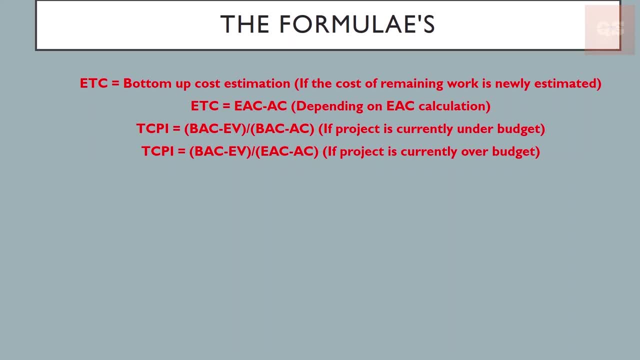 also, there are two scenarios. One is your bottom up cost estimation. So the bottom up cost estimation, that is, your newly freshly estimating your cost to carry out the remaining works. Another scenario is you are depending upon your estimated completion calculation based on, as I said earlier, there are 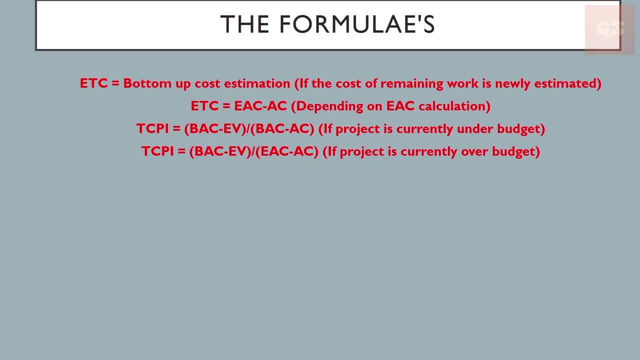 different ways of calculating your estimated completion. So based on that, your estimate to complete will be your estimated completion, depending on the different scenarios, which is your apt scenario minus your actual cost that has been incurred at the current stage. Now to calculate cost performance index, there are two scenarios. First one is in the current situation. if your project 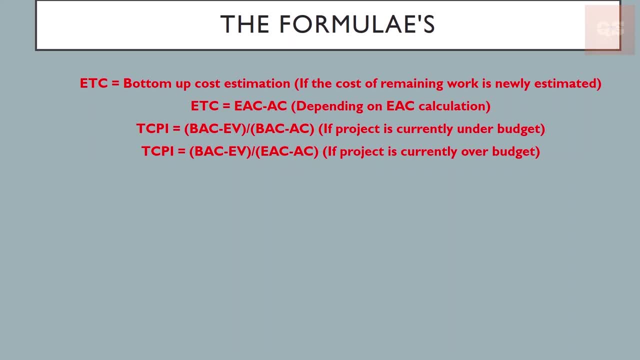 is under budget. So if that is a situation, then your to cost performance index will be BSE minus earned value by your budgeted completion minus actual cost. And in the current situation, if your project is over the budget, then your to cost performance index will be equal to the budgeted. 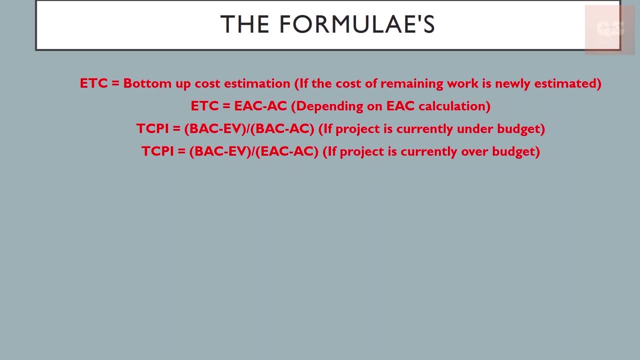 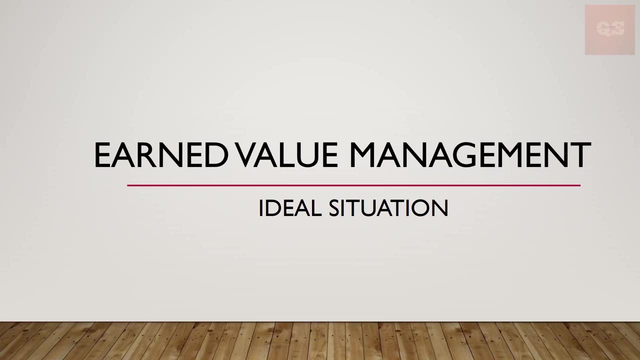 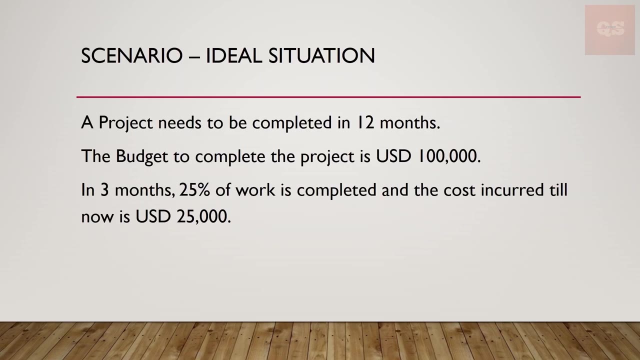 completion minus earned value divided by your estimated completion minus the actual cost. Now let's look at a scenario where you can understand earned value management concept more clearly. This is an ideal situation scenario. So this is the details of the situation. A project is needed to. 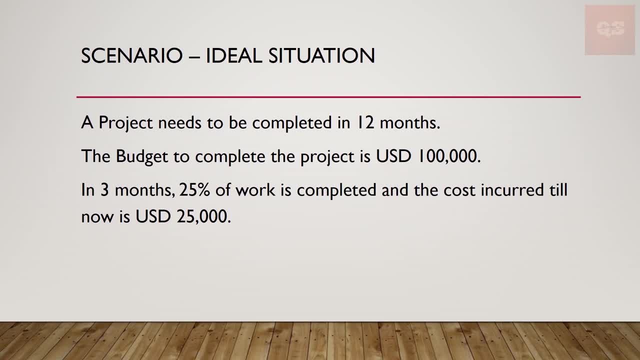 be completed in 12 months. The budget to complete the project is 100,000 US dollars, So in three months have been completed And in this three months 25% of work is completed And the cost that has been incurred till now is US dollars 25,000.. So let's see the calculations, how we can. 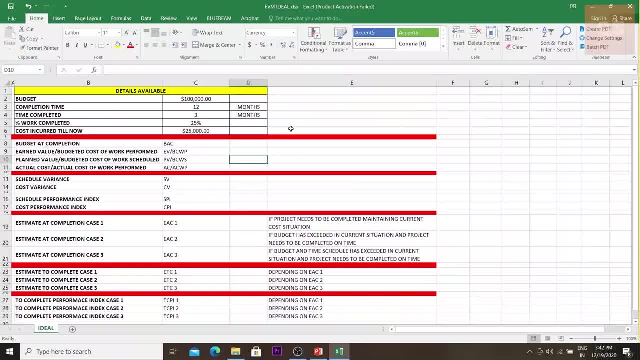 see the different components of earned value management in this situation. So these are the details that are available: the budget, the completion time, time that is completed till now, percentage of work that is completed and the cost that is incurred till now. So, from these, 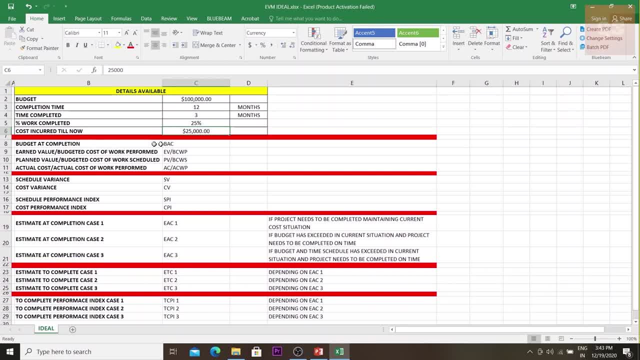 details. let's find out each component of earned value management. So your budgeted completion is simply equal to the budget which is given in the situation, that is, 100,000 US dollars. Now, earned value is the percentage of work completed into the budget. So now, 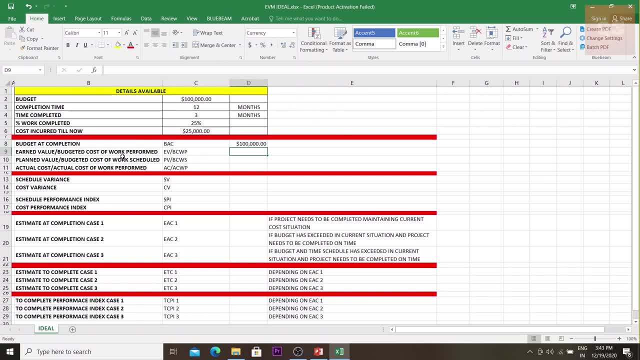 25% of work is completed. So your earned value will be 25% of your budget. that is, 100,000.. So this is simply equal to 25% into the budget. So your earned value is 25,000 US dollars Now. 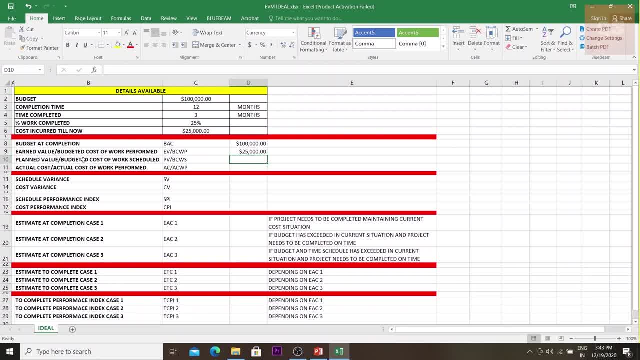 let's find out the plan value. plan value is the percentage of time completed into the budget. So right now the percentage of time completed will be three divided by 12.. So that is, three divided by 12 means 25%. So start. 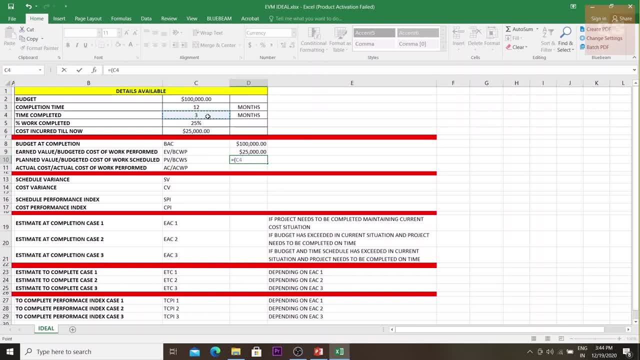 budget. so we'll calculate that. so your time completion is three divided by the total time, into make it into a percentage and then into that with the budget. so here 25 000 is your planned value and your actual cost is already given here. that is equal to the cost incurred till now: 25 000. 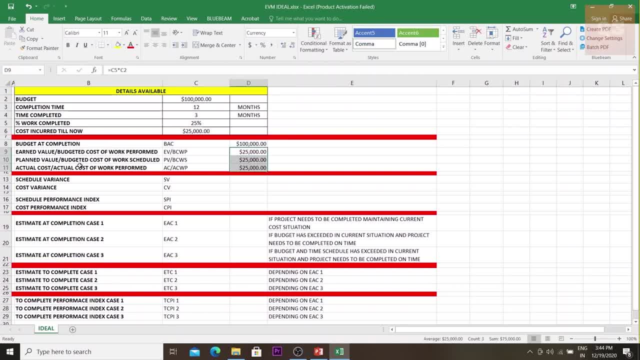 so in an ideal situation, you can see that your run value, plan value and actual cost are all the same. now let's find out the schedule variance. the schedule variance, as per the formula, is your earned value minus your planned value. so you've got zero. so zero means your project is on schedule. so 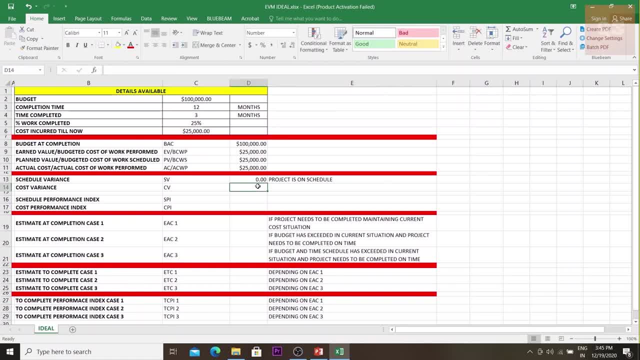 your project is on schedule. now we'll find out the cost variance, which is equal to the earned value minus the actual cost, which is again zero. so that means your project is on budget. now. finding out the schedule performance index: this is simply your earned value data divided by the plan value. that is one. so, since it is won again, the project is on schedule. your cost: 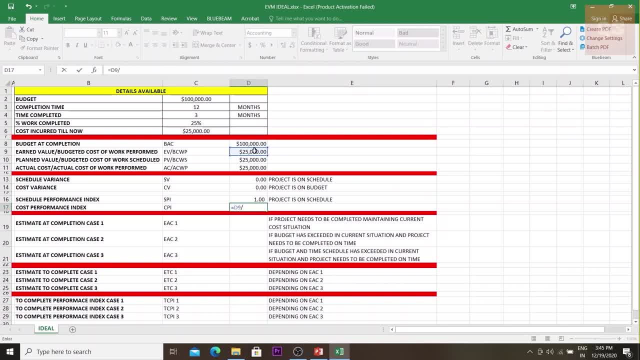 performance index will be equal to the earned value divided by your actual cost, again one. so that means project is on budget. now let's find out estimated completions. we have already seen there are different cases by which we can find out an estimated completing. the first case will be: 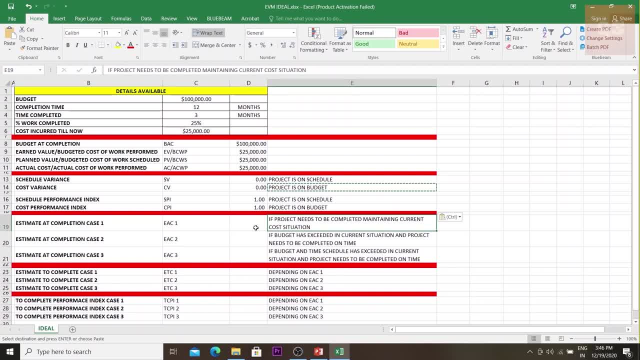 maintaining the same cost situation as of now. so in that scenario your estimated completion is simply equal to your budget period value and the cost of theancy is confirming the same around the end. so you see here a 4 undecided wait was given and the cost performance will be calculated with that. 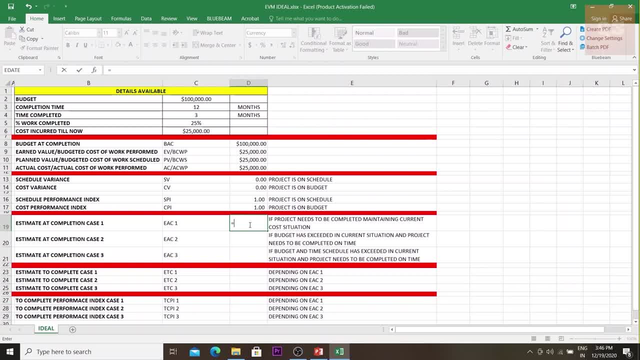 budgeted completion divided by your current CPA. so that is equal to your budgeted completion divided by your current CPA. so your estimated completion will be similar to what your budget is. since it is an ideal situation, you will be completing this project on budget. in the second case, it is when your budget has exceeded in the current situation and you need to complete. 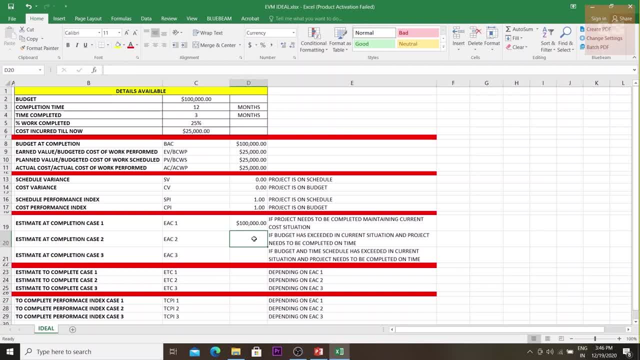 the project on time. if this situation is happening, your estimated completion formula will be equal to your actual cost plus your budget at completion, minus earned value. so this is this: formula will be used when, if at all, your budget has exceeded, since here, in this case, our budget has not exceeded. but just to show you the different scenarios, the different 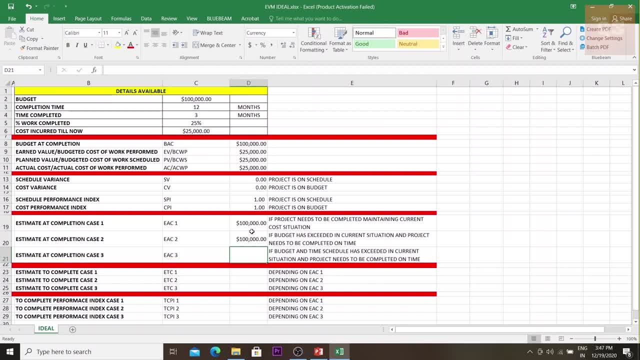 cases i have used in this formula again, when we calculate, you get hundred thousand as your estimated completion, and the third scene will be when your budget and time both has exceeded and you need to complete the project on time. if this is the scene, then your formula that you will be using will be your actual cost plus budget at completion, minus earned value. 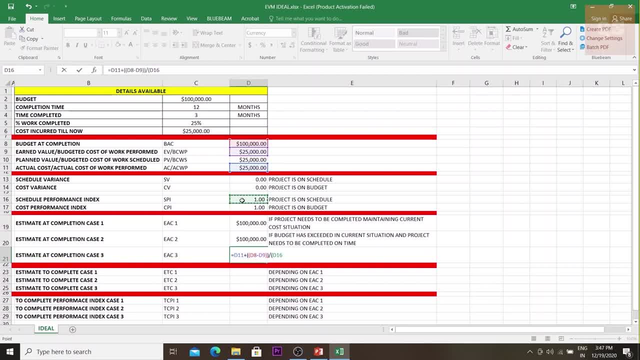 divided by the scheduled performance index into your cost performance index. okay, i've just put one bracket extra, so again you will get your estimated completion is hundred thousand. these are the three cases, depending on the situation of project, by which you can calculate your estimated completion. now again, estimate to complete. again here there are three cases based on your estimated. 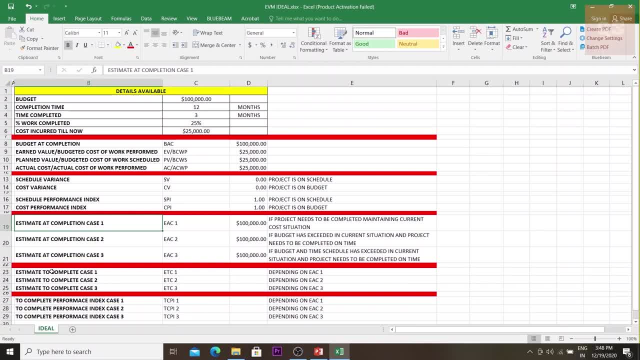 come how you have calculated your estimated completion. you need to find out your estimate to complete. so in the first case, if your project situation is to maintain the current scenario, then your estimated completion will be simply your. after finding out your estimated completion minus your actual cost. so you've incurred a cost of 25 000. so to complete the remaining work, you 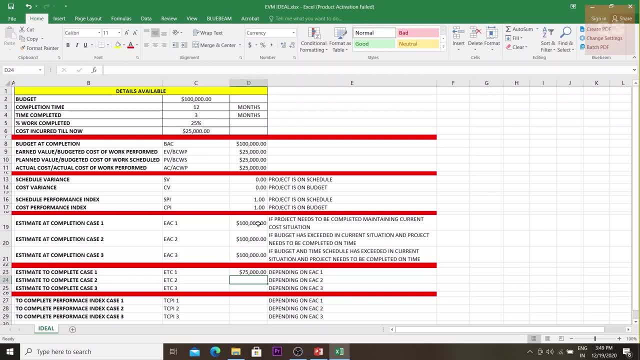 will be, you'll be, you'll be obviously needing 75,000 to reach 100,000 of budget. So if you're using, if it was a second case, then again similarly, your estimated completion minus your actual cost, Here again it is 75,000. and if it is a third case, 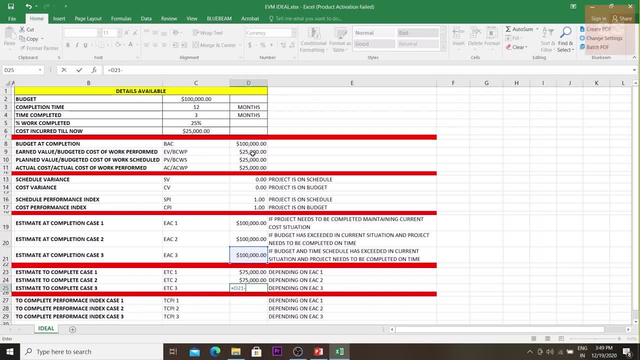 the third way how we will find out the estimated completion minus your actual cost. So in all, since this is an ideal situation, your estimate to complete will be 75,000 in all three cases. Now we'll find out again the total to complete. performance index. 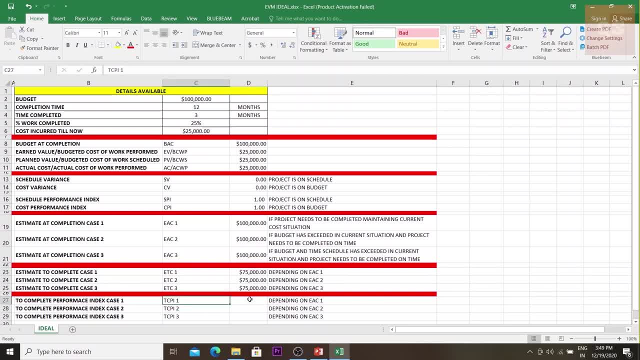 This again based on how you have calculated your estimated completion. we'll be using the formulas. So here, the first case, since our budget is cost has not exceeded, the formula that you will be using will be your budget at completion minus earned value. 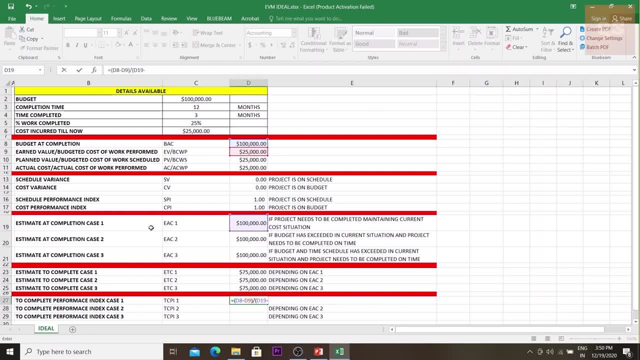 divided by estimated completion. estimated completion, that is calculated in the first case minus the actual cost. So this is the formula. since your budget has not exceeded, this will be your formula. So in the second scenario, if you're using this calculation, 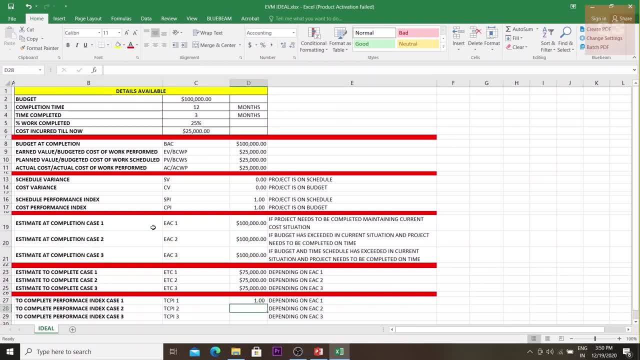 this is the scenario. Again, the formula will be similar, except your estimated completion. you will be using this part, So it is equal to budgeted completion minus earned value divided by your estimated completion minus actual cost. And the third scenario: again, your budgeted completion minus earned value divided by 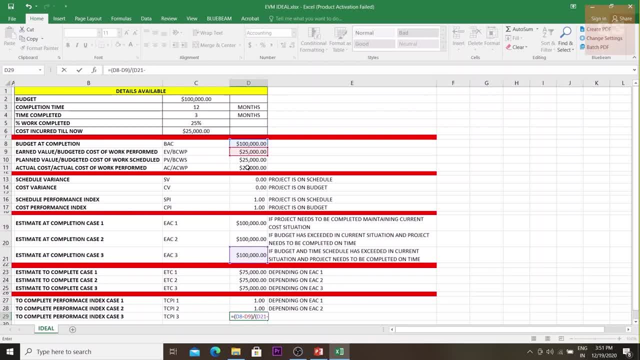 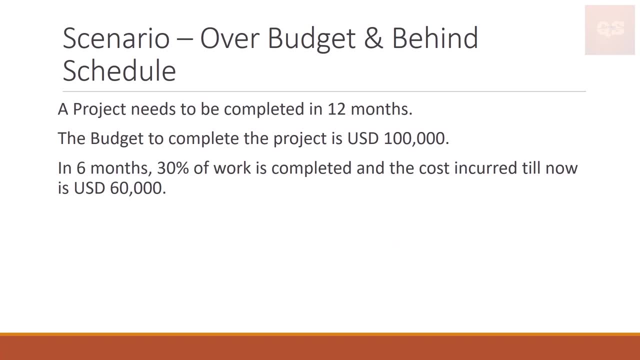 your estimated completion. this scenario minus your actual cost. So hope this ideal situation scenario is clear and how you've calculated different earned value components. Now let's see an example where your project is over budget and behind schedule. So your project is needed to be completed in 12 months. 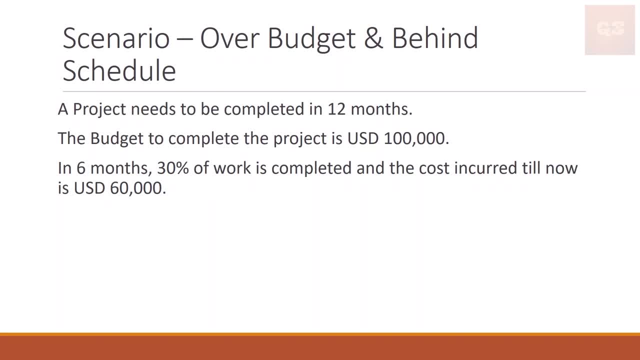 and the budget is 100,000 US dollars. So six months have been completed and, in the current situation, 30% of your work is completed and the cost incurred till now is 100,000 US dollars- 60,000.. 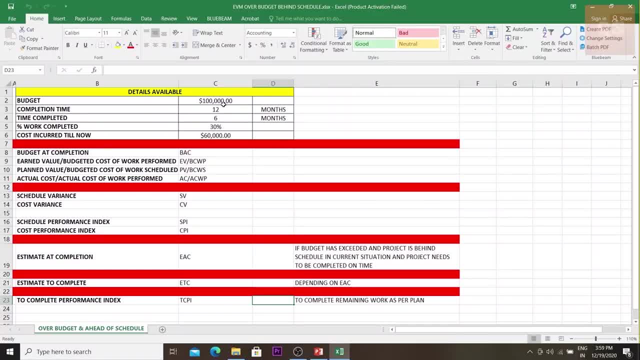 So this is a scenario. So let's see the calculation. So these are the details available. Your budget is 100,000 US dollars. The completion time is 12 months. The time completed till now is six months. The worst percentage of work completed is 30%. 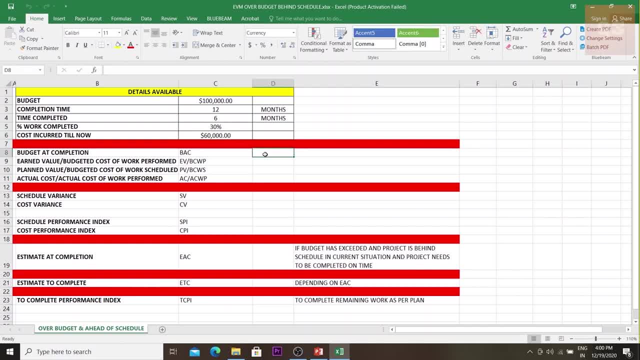 and the cost incurred is 60,000 US dollars. So from here the budgeted completion is similar to your budget: 100,000 US dollars. Your earned value will be your percentage of work completed into your budget, So that means your 30% into 100,000.. 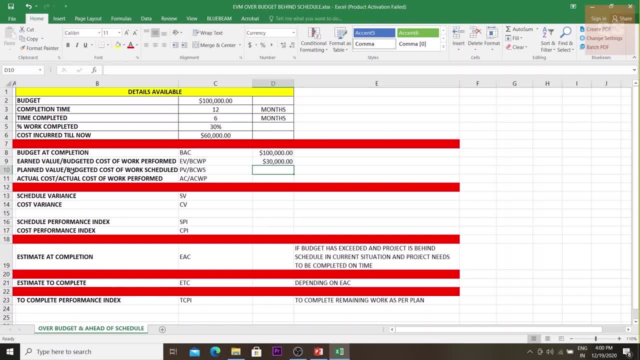 So 30,000 US dollars is your earned value. Your planned value will be the percentage of time completed into the budget. So here first, to find out the percentage of time, it will be six divided by 12 into 100 percentage into your budget. 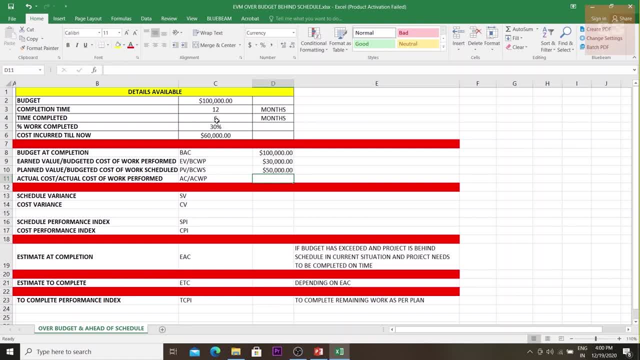 So 50,000 is your planned value because, since half of the period is completed as per plan, you must have incurred around 50% of the budget, that is, 50,000.. So that is what we have got here. Your actual cost is equal to what? 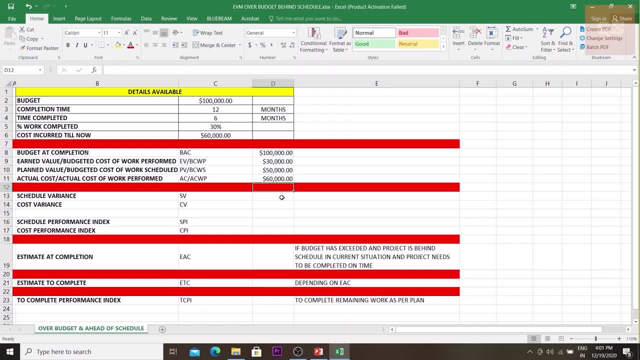 Your cost incurred is, so, that is, 60,000 US dollars. Now let's find out the schedule variance and the cost variance. Schedule variance is equal to earned value minus planned value, So the value that you got is negative, which means that your project is behind schedule. 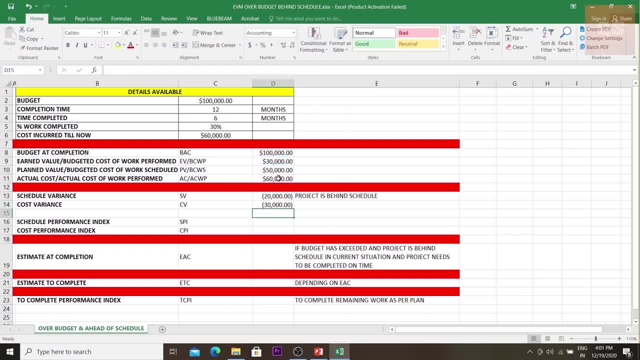 Your cost variance will be your earned value minus your actual cost. So again, the amount that you got is negative means your project is over budget. Now we'll find out the ratios. The schedule performance index will be equal to earned value divided by planned value. 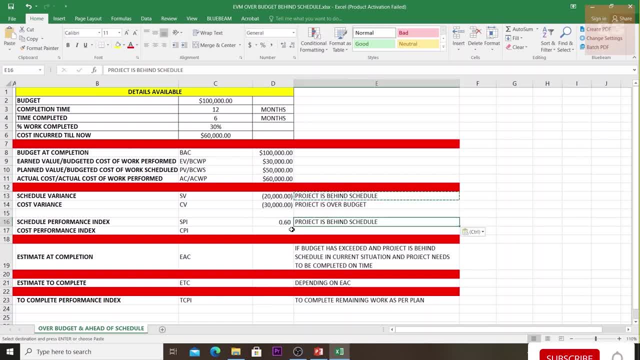 So 0.6, it is less than one. So again that means the project is behind schedule. Your cost performance index will be earned value divided by actual cost. So 0.5, that is less than one- means your project is over budget. 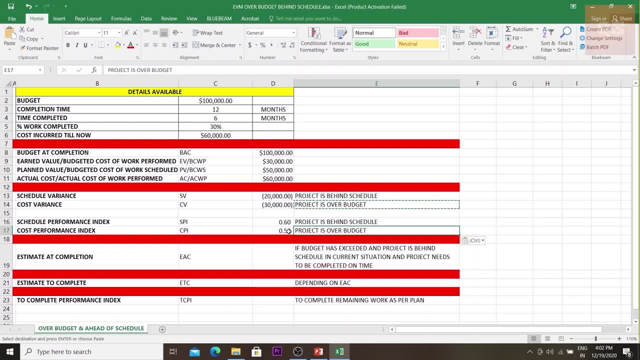 This means that for $1 that you spend, you will be earning 0.5 US dollars. So that is the meaning of cost performance index. So every one US dollars that you're spending, you will be earning 0.5 US dollars. 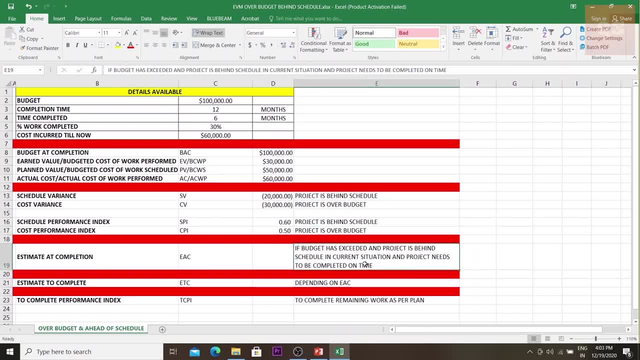 So now we'll calculate the estimated completion. So, since the budget has exceeded and the project is behind schedule, so in this scenario, if you need to complete the project on time, the calculation, the formula that you use for calculating your estimated completion, will be: 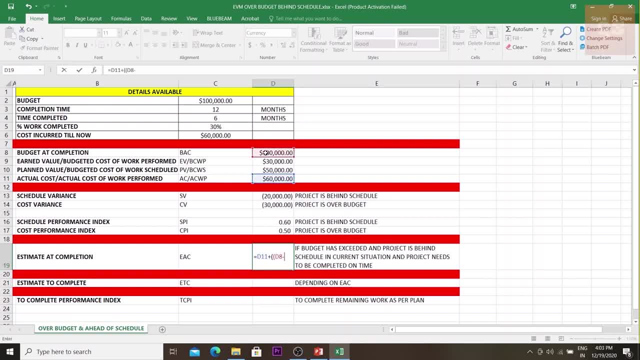 your actual cost plus your budgeted completion, minus earned value, divided by the schedule performance index into your cost performance index, So you'll get an amount 293.5.. So this is going to be your final estimate at completion set. You started your project with a budget of 100,000,. 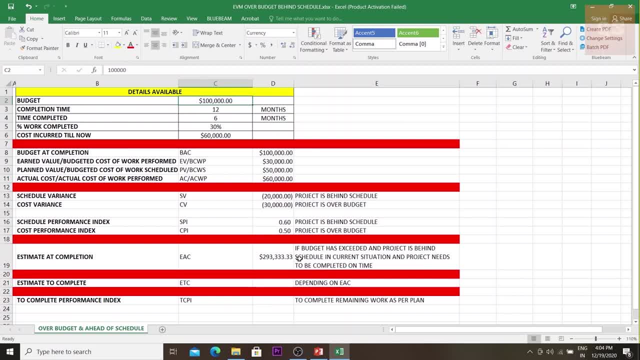 but once you complete your project, because of these current situations, you'll be spending around 293,333.33 US dollars, So your budget for completing this project is going to be this much. So, in this situation, your estimated completion- sorry, your estimate- to complete. 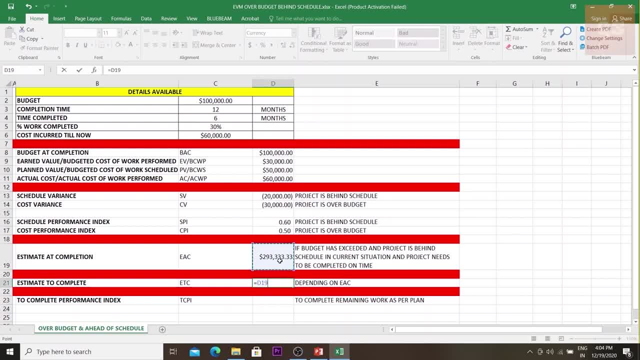 that is, to complete your remaining work, is going to be your estimated completion minus your actual cost To carry out the remaining works, you'll be incurring a amount of 233,000, because 60,000 you've already incurred. And finally, to complete the remaining works, 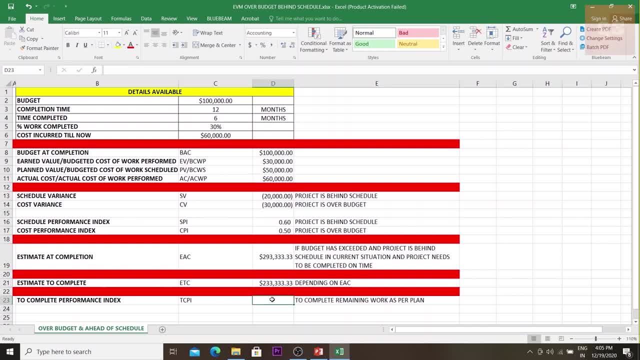 as per the plan. that is your future cost performance index, Since your budget has exceeded the formula which you're going to use here is the budget at completion minus earned value, divided by estimate at completion minus your actual cost. So 0.3 will be the cost performance index. 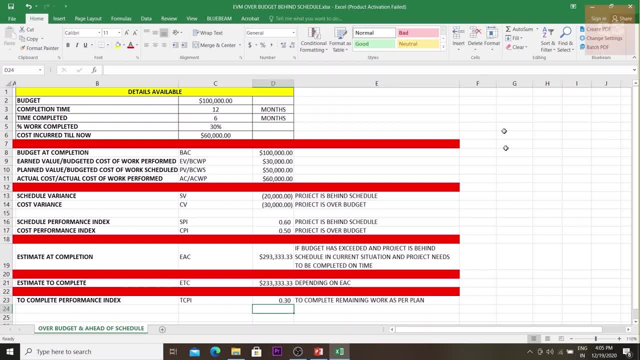 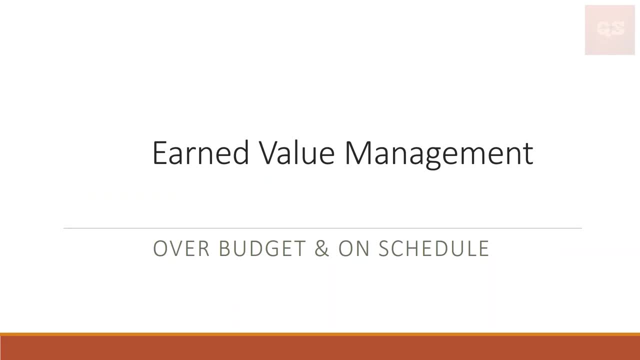 to complete your remaining work as per plan. So hope the situation is clear now and how we have calculated the different components of earned value management when your project is behind your schedule and the project is over the budget. So now we'll see a scenario where your project is over budget but on schedule. 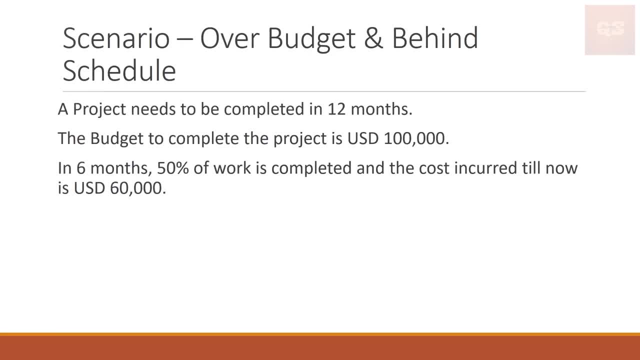 So this is the situation. Your project needs to be completed in 12 months. The budget is 100,000 US dollars, So six months is over and 50% of your work is completed, And the cost incurred is, till now, is, 60,000 US dollars. 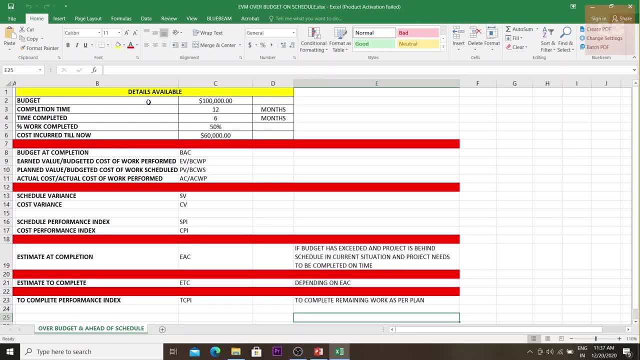 So let's see the calculations. So these are the details that are available: Budget completion time, time completed till now and the percentage of work completed plus your cost incurred till now. So your budget is already given as 100 US dollars. 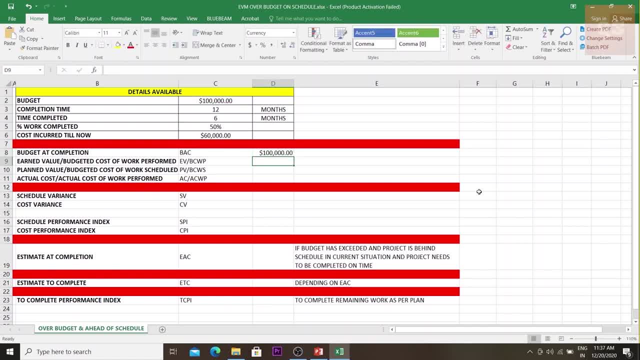 100,000 US dollars. Your earned value will be your percentage of work completed into your budget, so 50% into your budget. Your planned value will be your percentage of time completed into the budget. So that will be equal to six divided by 12. 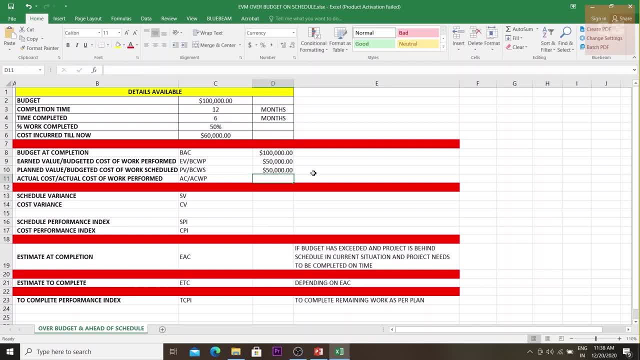 into 100 percentage into your budget. It is 50,000 US dollars and your actual cost is already given as 60,000.. So now we'll find the schedule variance. The schedule variance is earned value minus planned value, So that is zero. 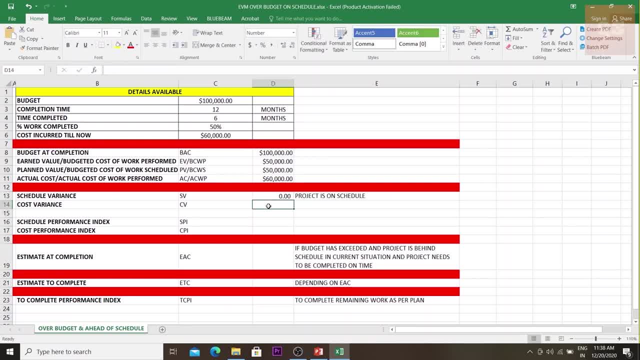 So zero means your project is on schedule And we'll find the cost variance is equal to earned value minus actual cost. So it is a negative value. That means the project is over the budget. We'll find the schedule performance index That is equal to earned value divided by planned value. 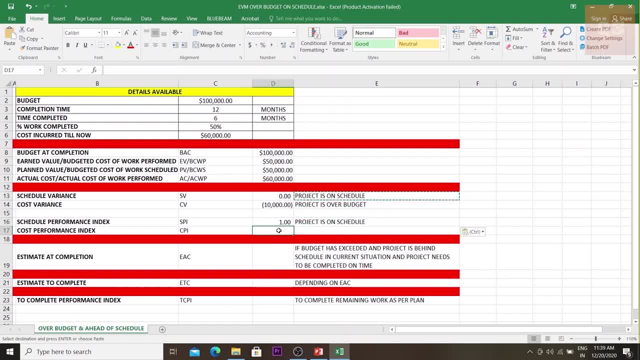 This is one. So again, that is project is on schedule And your cost performance index is earned value divided by actual cost, So that is less than one. That means it is project is over the budget. Now, since the project is over budget, 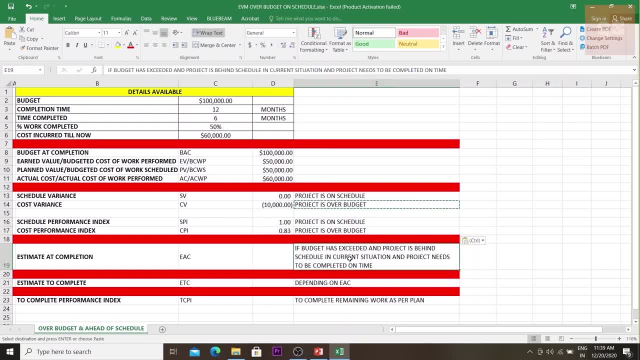 and so this situation situation is: if budget has exceeded and project, the project is on schedule. here, project is on schedule and project needs to be completed on time. So if this is the situation, you need to use the formula that is actual cost. 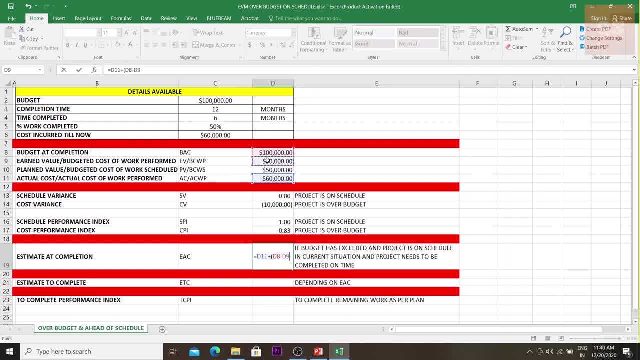 plus your budgeted completion, minus earned value. So finally, your estimated completion is going to be 110,000 US dollars. Your budget initially was 100,000 US dollars, due to the current scenario where your cost incurred is above the budget. So finally, when you complete the project, 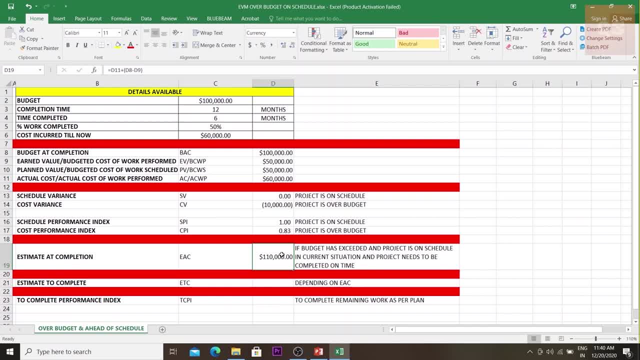 at the time of completion of the project, your cost is going to be 110,000 US dollars. Your estimate to complete is going to be your estimated complete minus your actual cost. So, to complete the remaining work, 50,000 US dollars will be spent.